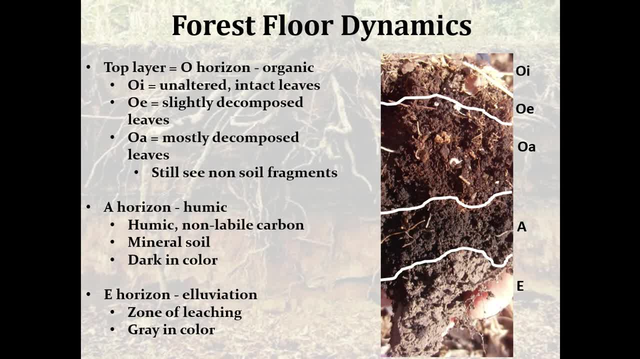 the way down to mostly decomposed leaves. but we're not seeing any mineral content until we get to the A horizon. That's where we have our humic non-layable carbon. We'll get into what that means more later, but it's a mineral soil, dark in color. Our E horizon. 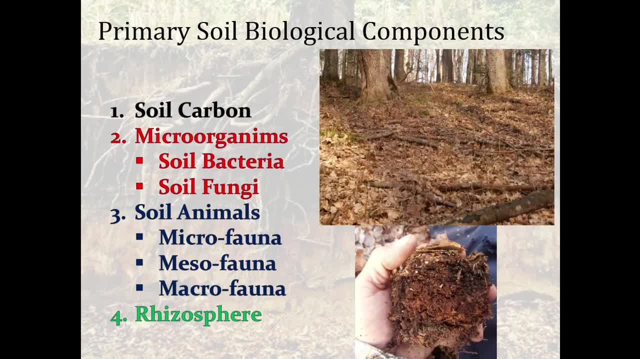 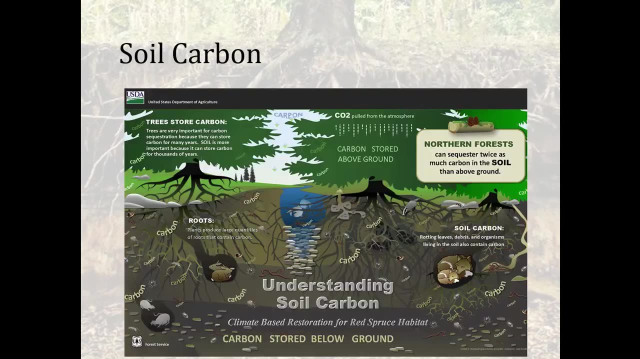 zone of leaching, usually lighter in color, often gray. So primary soil biological components is the soil carbon, then our microorganisms, our macro organisms of our soil animals, and then we will talk about the rhizosphere. So soil, carbon Soil. 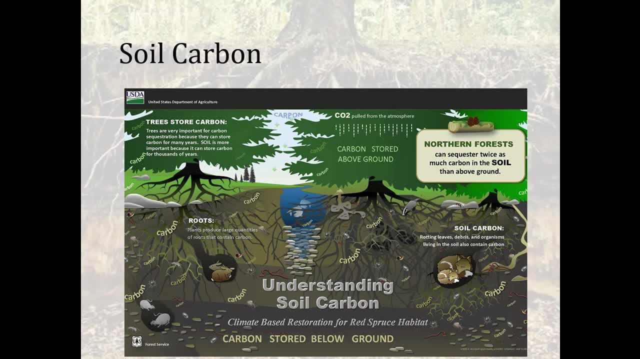 carbon drives our nutrient availability for plants and animals, the importance of forests in the role of our session, and then these carbon NH levels through our soil contain a very high. seriously, Пока, però, we'll go with soil carbon. we'll get into that in just a pretty minute. So soil carbon is a greatла Mikey's about of the cofinancial blocks for plants and animals. but So soil carbon can also live significantly longer than water they can. they became layerically if warmed over a 10 to 9 kgIT per day top of the food. So you can see from the various parameters here. 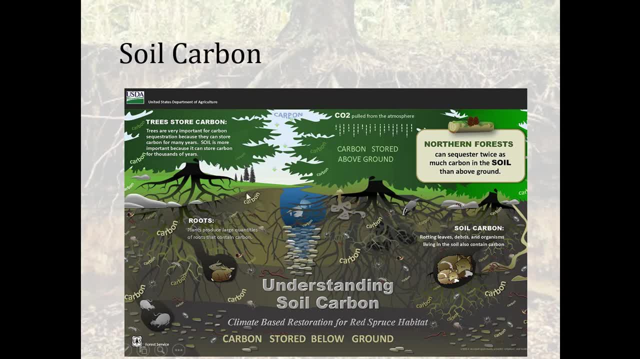 always three. heute viatásavaro i this river to ensure that the permac household of soil carbon. A little note here that forests are able to sequester twice as much carbon below the soil than they are above it. so a lot of times we think oh. 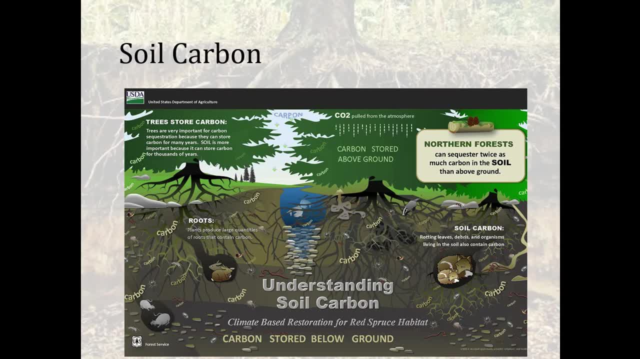 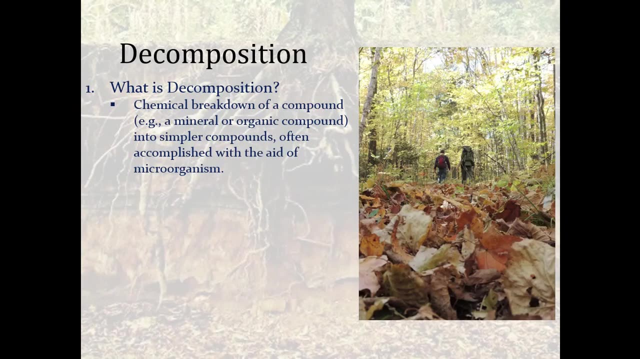 we need to grow more trees, grow forests, stop cutting down our forests. but it's really their ability to store that carbon in the soil for long-term cycling down there. that is also really important when it comes to carbon sequestration. So, decomposition of organic matter First. we start with what is decomposition. So 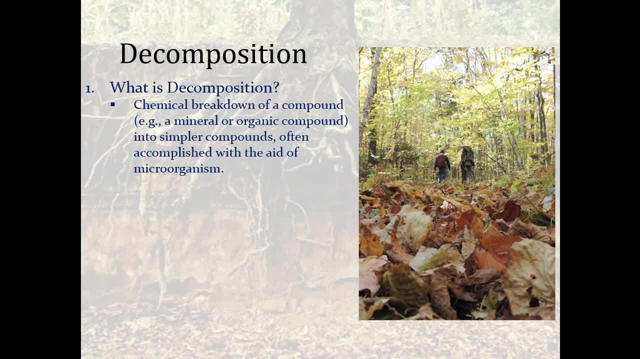 it's the breakdown of a compound into simpler compounds, So I think of like a really long carbon chain. when it gets decomposed it forms like two shorter chains, and so on and so forth. It's a simplification of structures, often for the gain of microorganisms. 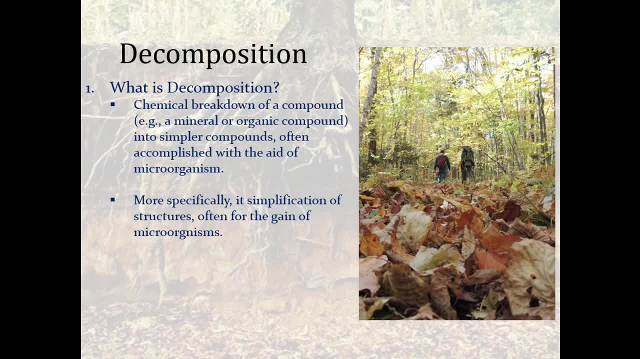 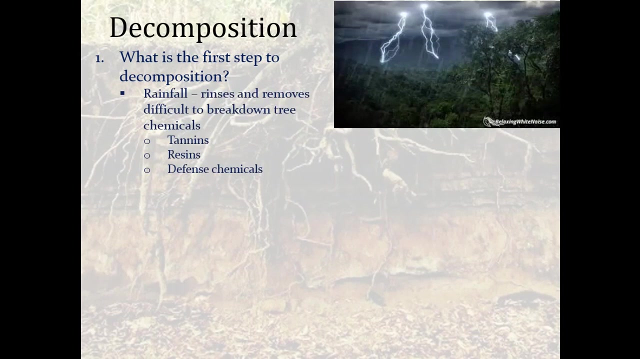 Eventually, these microorganisms decompose to the point that the plants can then use those nutrients again as well. So does decomposition only occur from living organisms? We will find out. The first step of decomposition, Rainfall. So there's our answer: Rainfall, not a living organism, but really important for 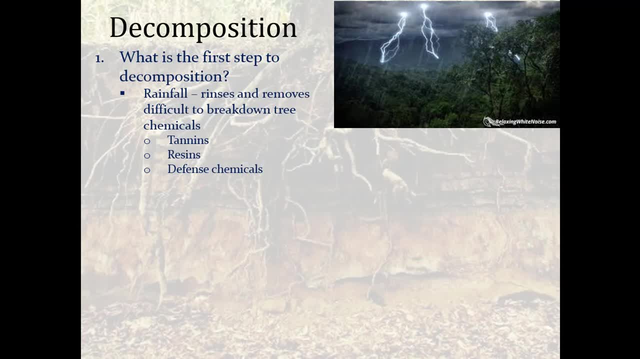 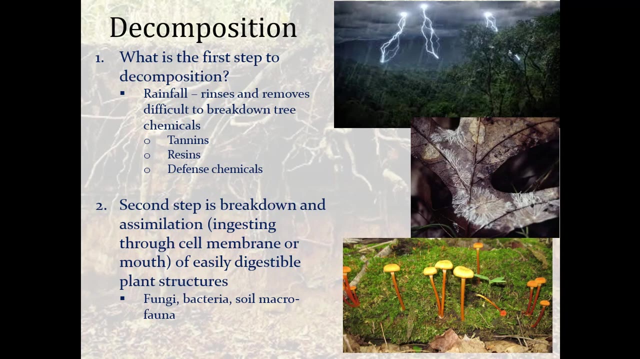 decomposition for the material to get wet, as well as rinse away certain of those tannins and other defense chemicals from the tree components, especially the leaves. then the second step is assimilation or the ingesting of a cell membrane through a mouth or easily digestible plant structures. so fungi, bacteria, soil macrofauna are 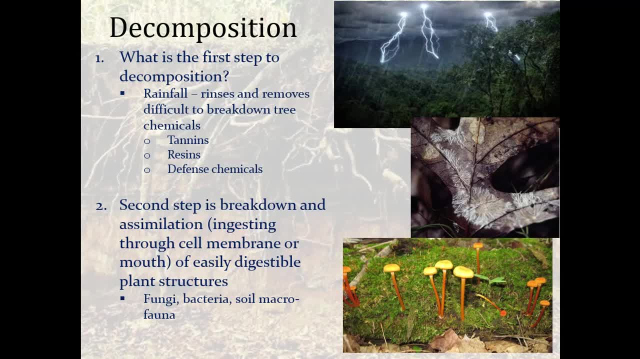 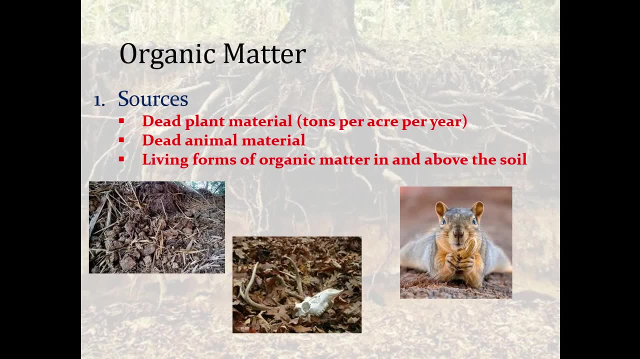 beginning to break down the cell membrane and break those long carbon chains into shorter components. sources of organic matter probably most often think of dead plant material, so this is just naturally cycling material. we also have dead animals in there in a more natural setting- think of those carcasses- and things come to feed on them. but there's always some part of it. 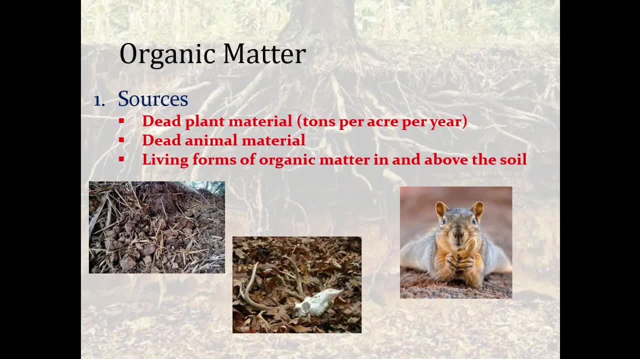 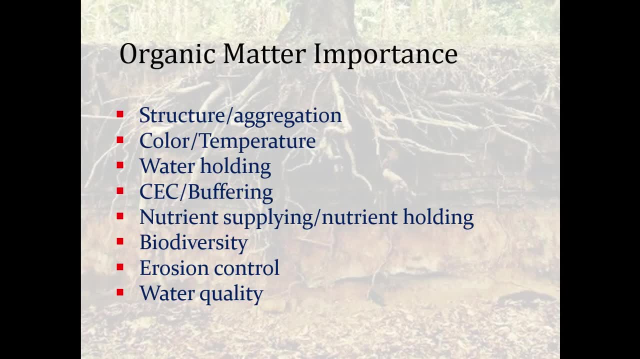 left in the soil or from animal waste that is being broken down, and then there's living forms of organic matter in above the soil. this would be our plants. the importance of organic matter- we mentioned it in some previous videos- for soil structure and aggregation, color, water holding capacity, cation exchange capacity or nutrient supply. 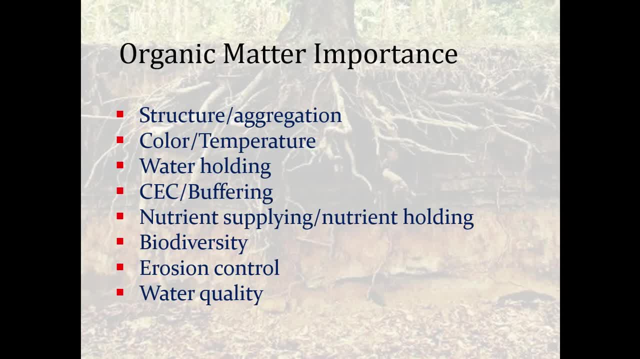 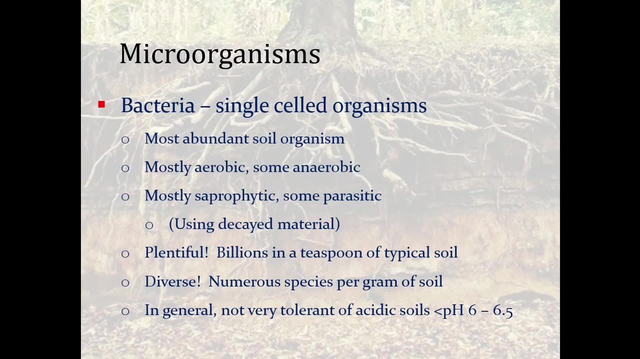 and holding biodiversity in our micro and macro organisms and plant communities, and then both of those drive erosion control and water quality. so water filtering as well microorganisms are. we have our bacteria, which are single-celled organisms. these are the most abundant soil organism, mostly in aerobic conditions. some do operate better in. 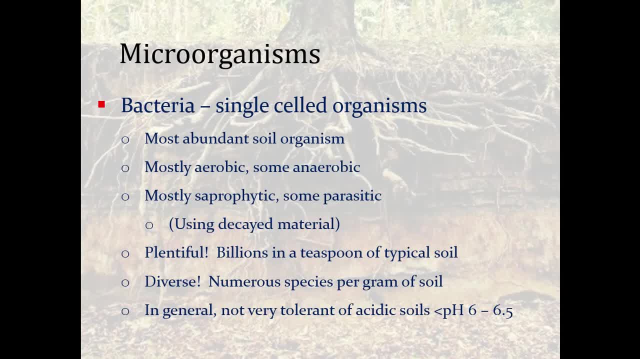 anaerobic, remember. aerobic means in the presence of oxygen. anaerobic is when there's a lack of oxygen available. but some are parasitic, and here a reminder that saprophytic means that they use decaying material. parasitic would mean that they feed on living. 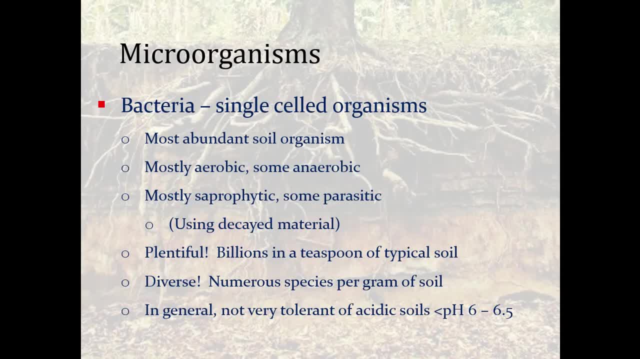 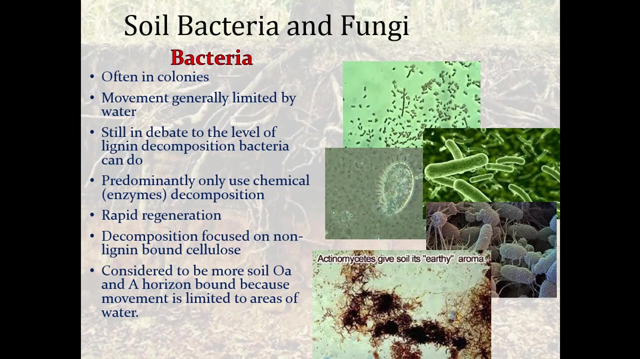 material bacteria are incredibly plentiful and diverse in the soil but in general not very tolerant of acidic soils. so as we get below pH of six and a half to six, we lose a lot of our bacterial communities. while they are single-celled organisms, they often form colonies and move through the use of 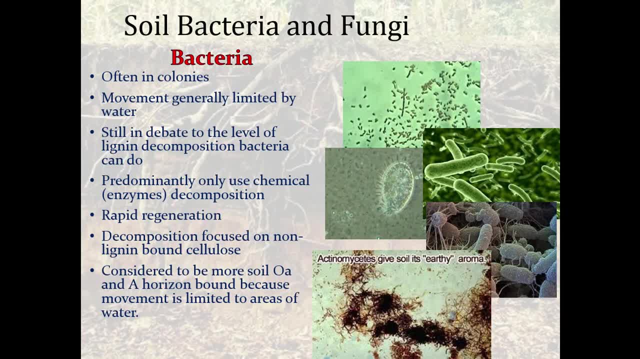 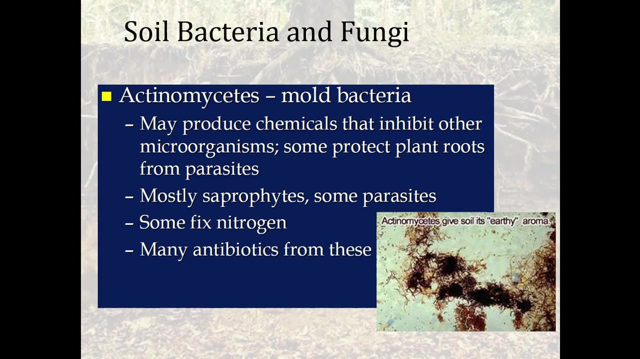 water. they predominantly use chemical decomposition and feature rapid regeneration. so when conditions are right, your bacterial population can quickly grow and sort of use all of those conditions that favor them. you mostly found in, like the OA a horizon, because their movement is limited by water, actinomycetes or mold bacteria. it's just one subcategory bacteria, but 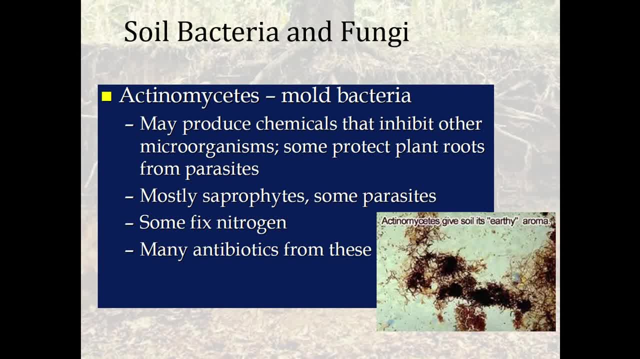 we highlight it because it produces chemicals that inhibit other microorganisms. some of those chemicals then protect plant roots from parasites, so sort of a symbiotic relationship going on here. these are also some of them that fix nitrogen in the soil. and then many antibiotics come from mold bacteria and we talked about in the intro video the 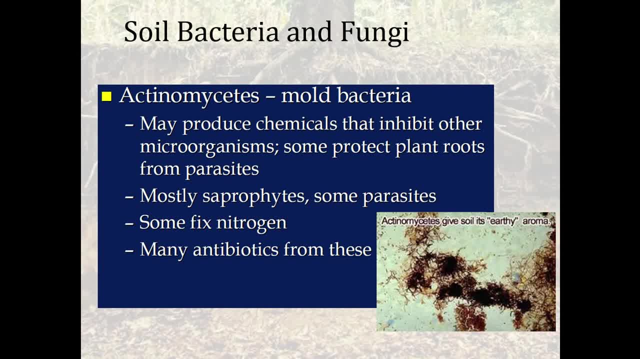 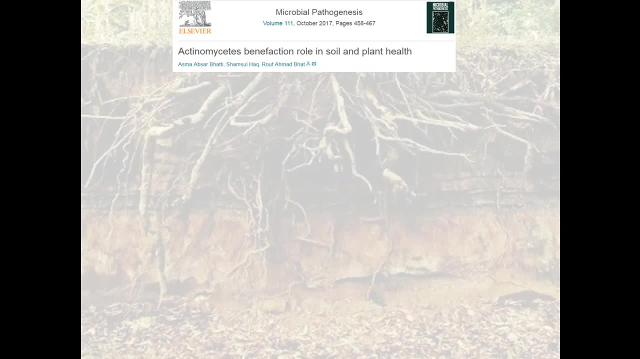 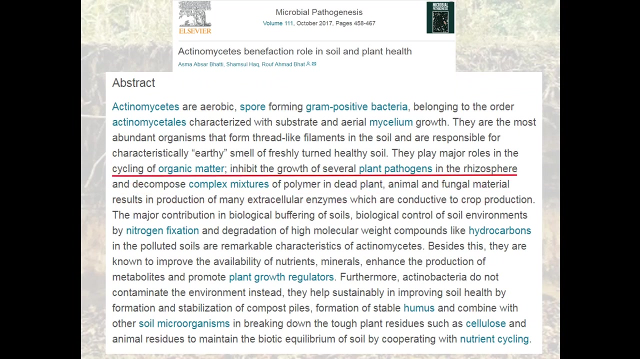 importance of soil bacteria for development of pharmaceuticals. so this is a family that they research and look for and test for future drug development. so if you want more reading, here's a really good paper on. you know my CDs beneficial benefit in soil and plant health and just highlight cycling of. 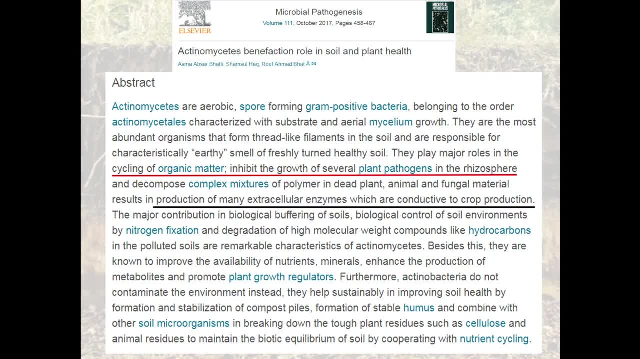 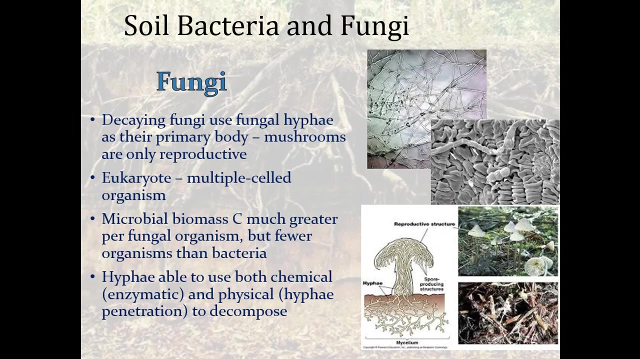 organic matter, inhibit several plant pathogens, improve crop production and then improve availability of minerals, nutrients and metabolites for plant growth regulators, as well as form stable humus, and we'll talk more about humus in a later video. we also have fungi in the soil, so decaying fungi use. 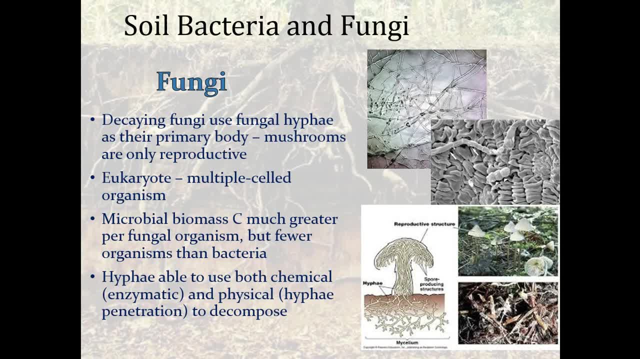 hyphae as their primary body. these are sort of like roots- it's easier way, or easy way to think of them, although they function differently- but sort of these root structures in the soil. and then when I think of fungi, we always think of the mushrooms or, you know, shell fungus, things like that. but these are. 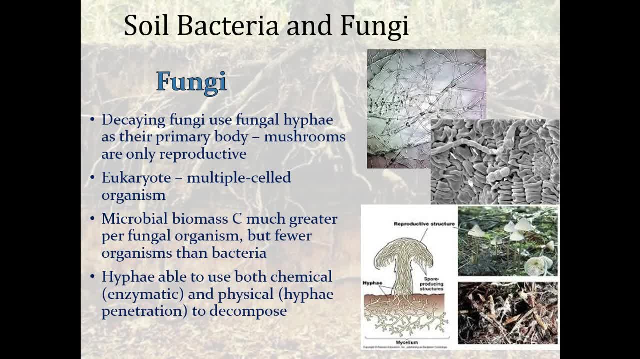 really just the reproductive body parts of them, and so a lot of times there's more mass below the soil that we're not seeing. so there's something to keep in mind. they are a eukaryote, or multiple cell organisms. the carbon is much greater per fungal organism, so an individual organism is much larger. but 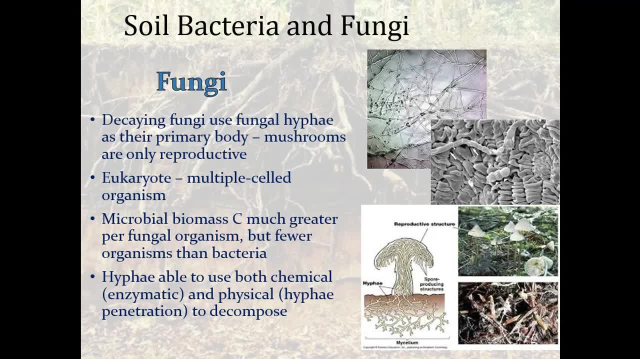 But the flip side of that is that there are fewer organisms than bacteria. If you think of bacteria, you know a single-cell organism forming a colony. That colony can be large, but that organism itself is sort of limited to that single cell. 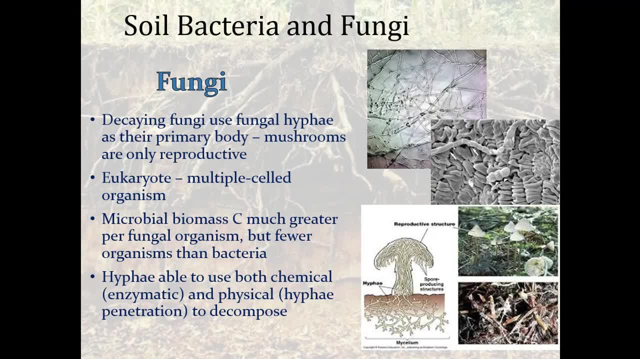 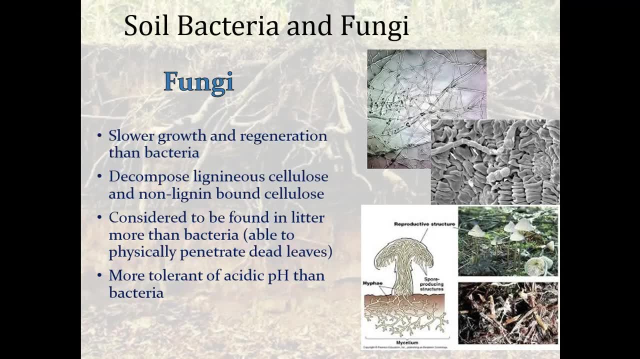 Fungi are also capable of both chemical and physical decomposition, So they can penetrate materials using their hyphae. Slower growth and regeneration than bacteria, but more longer-living, And they can decompose both lignin and non-lignin-bound cellulose. 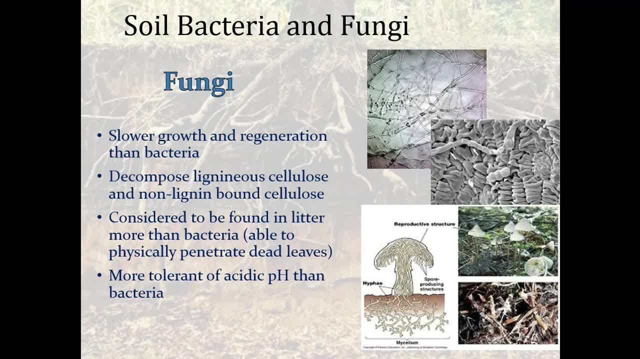 considered to be found in litter more than bacteria. So again, they're able to penetrate dead leaves, They're able to spread broader and deeper in the soil profile, as well as being more tolerant of acidic pH than bacteria. So a lot of times our forests are fungal-dominated due to that long, slow growth.